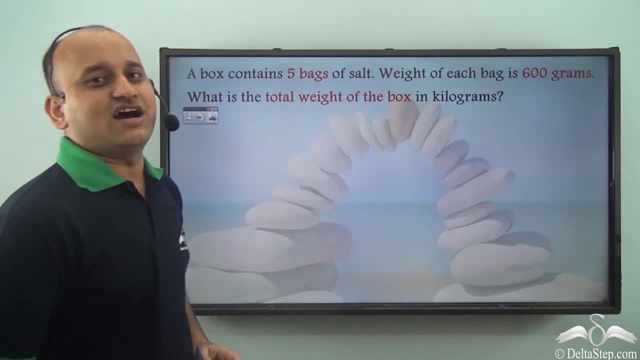 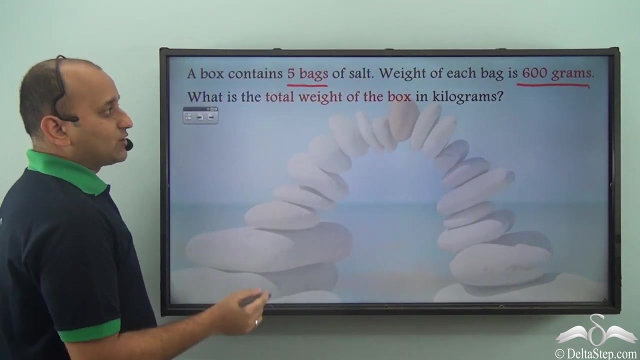 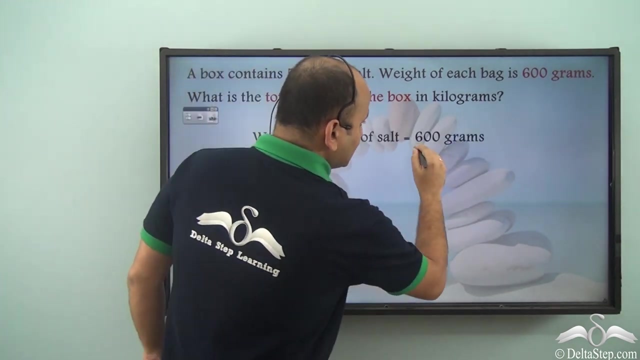 Weight of each bag is 600 grams. So what is the total weight of the box in kilograms? So what do we know? We know that there are 5 bags and each bag weighs 600 grams. So we need to calculate the total weight in kilograms. Now. weight of 1 bag of salt is 600 grams. So total weight of 5 bags of salt is 600 grams. So total weight of 5 bags of salt will be 5 into 600 grams. It is simple, which means 3000 grams. So the total weight in grams is 3000 grams. Now we need to calculate in terms of kilograms, isn't it? So we know. 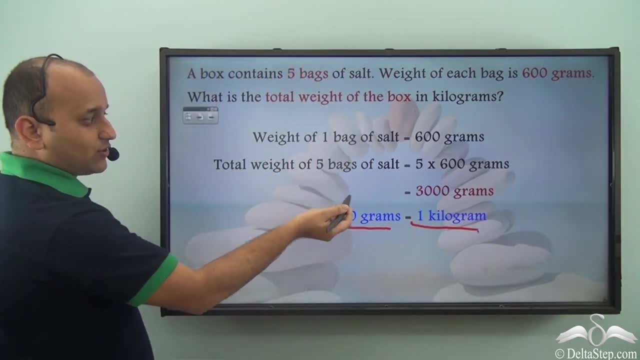 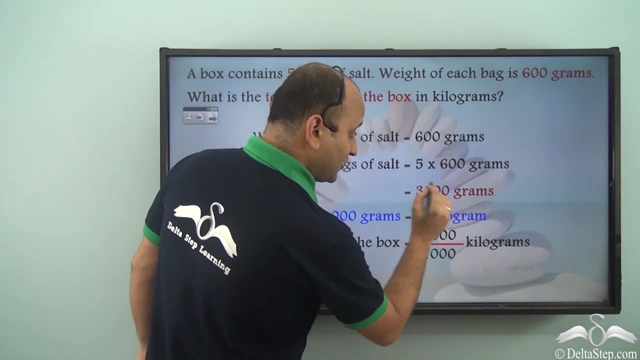 that 1000 grams is equal to 1 kilogram. So we are calculating for 3000 grams. So total weight of the box we are converting from 1 kilogram to 1000 grams. So we are calculating. We are converting from grams to kilograms. that is, smaller unit to larger unit. 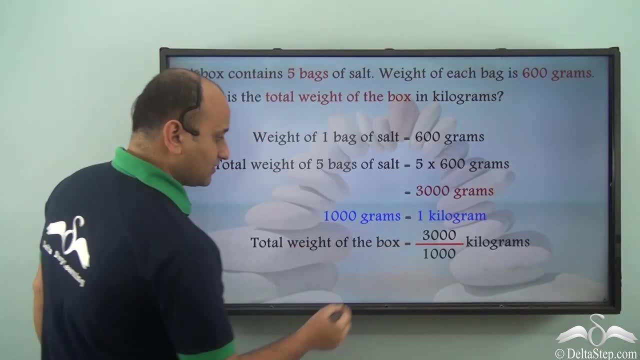 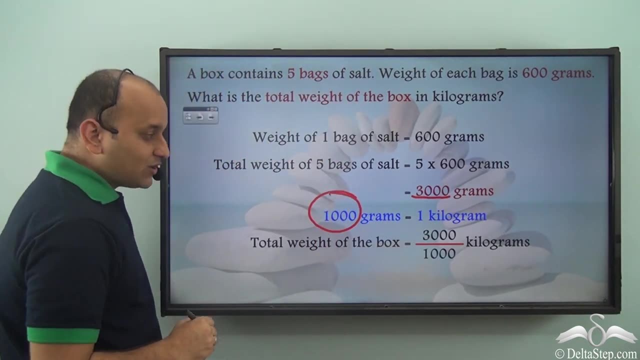 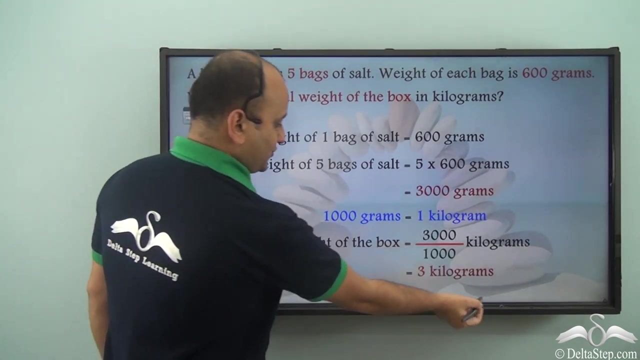 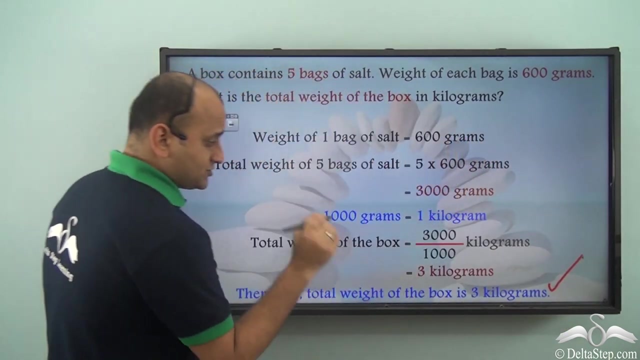 So we divide right. So we will divide 3000 by the conversion, that is, 1000 grams is equal to 1 kilogram. So it will be 3000 by 1000 kilograms, which is 3 kilograms. Therefore, total weight of the box is 3 kilograms. 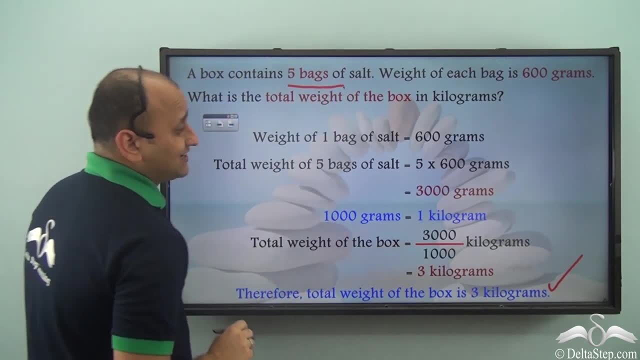 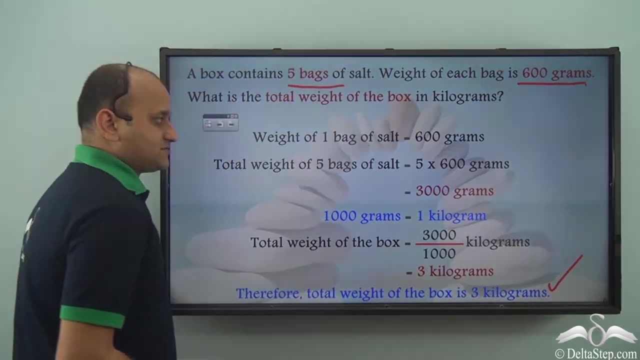 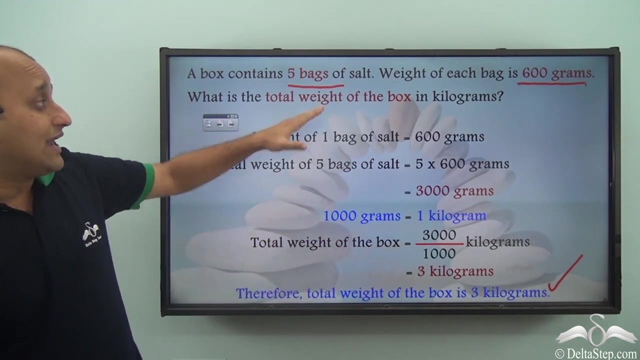 So you see, we had 5 bags of salt in the box and each bag weighed 600 grams, So the total weight is 3 kilograms. So by using this conversion rate, 1000 grams is equal to 1 kilogram. we were able to calculate. 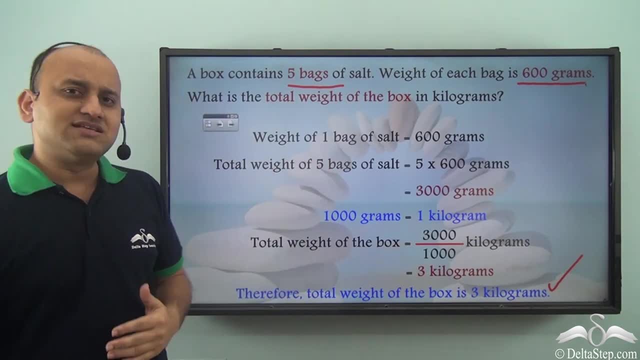 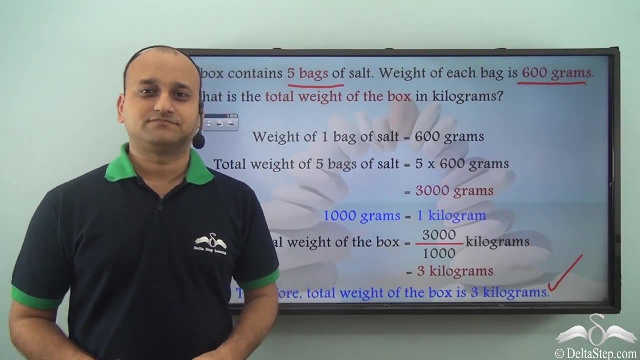 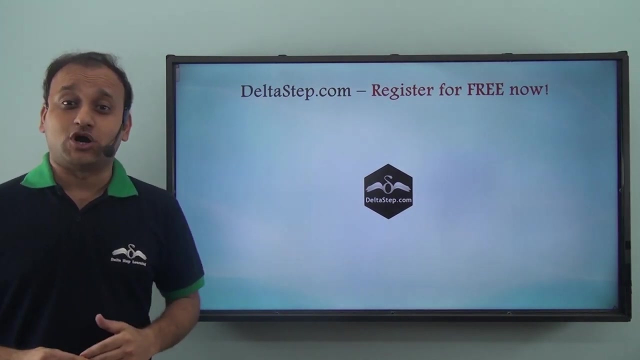 the total weight of the box. Similarly, you can apply the same knowledge in a number of word problems And you can practice more problems till you become perfect. Don't forget to subscribe to our channel. You can also register for free at deltastepcom to get all learning resources as per ICSE. 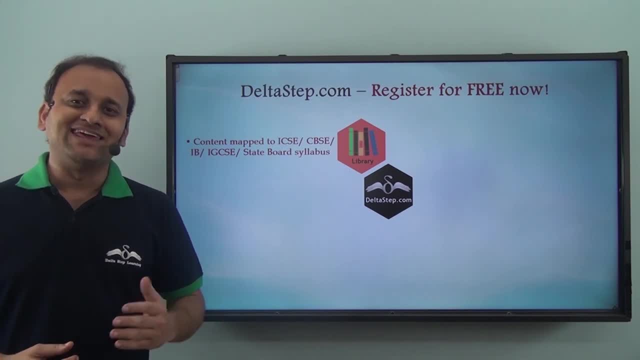 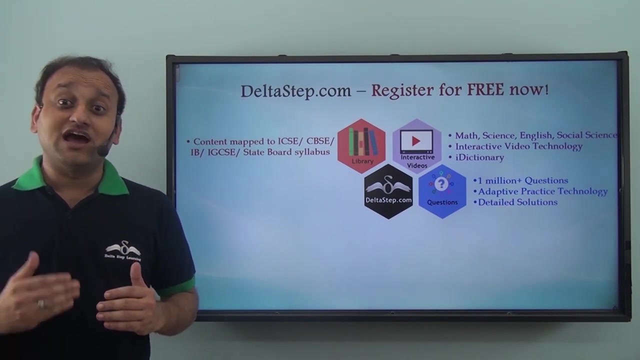 CBSE, IB, Cambridge or any other curriculum. Over 5000 amazing lectures across Maths, Science, English and Social Science. Our unique interactive video technology Keeps you engaged and our iDictionary feature allows you to quickly revise any concept. Master each topic at your own pace with our adaptive practice technology and 1 million.